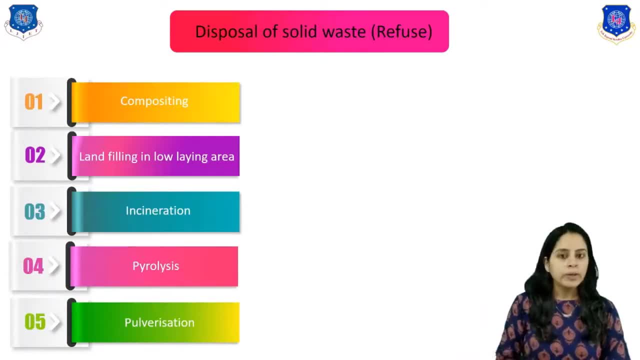 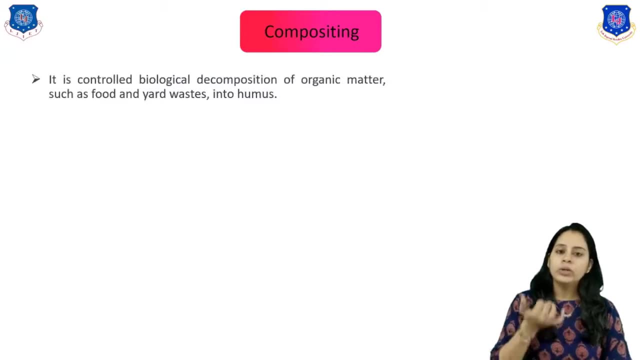 method and the last one, which is the pulverization. okay, So start with the first method, which is composting method. okay, So what is composting? right? So it means that it is a controlled biological decomposition of organic waste, such as food, vegetables, then house. it is arising from: 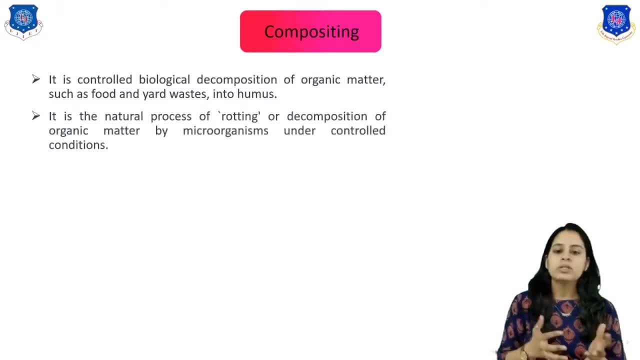 the household activities. Right, So it is a natural process of the rotting or decomposition of the organic matter by the microorganism under the controlled condition. right, So it can be aerobic and anaerobic also. right, And this process take a 4 to 6 week and the end product of composting process is called. 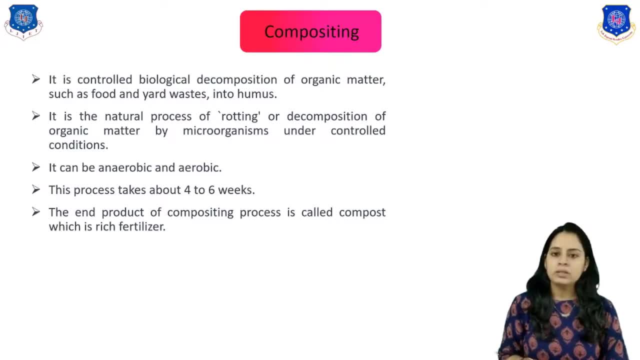 compost or which is which is rich fertilizer right. So the advantage of this method, which is it provide a nutrient to the soil, right, Because here, in this method, we are using organic waste right. So the it is increase the beneficial for the soil organism, then it protects soil. 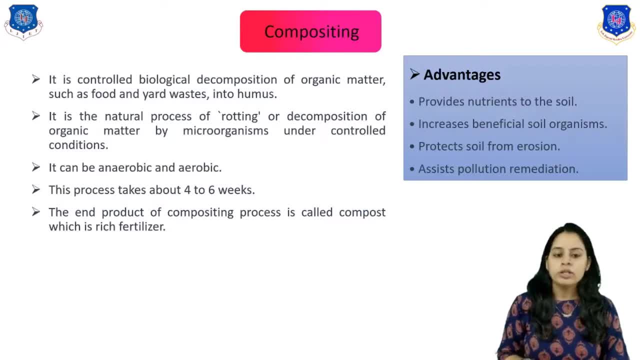 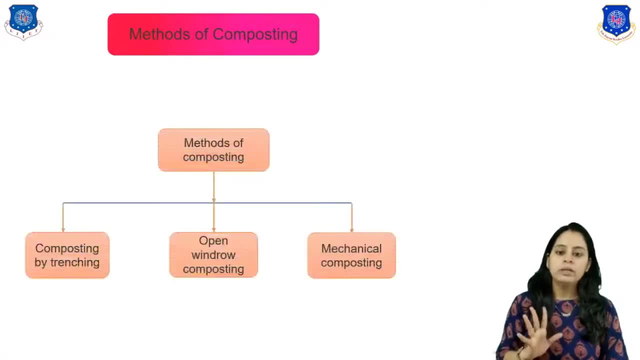 from erosion, then it assist for pollution remediation. right Now for the composting there are again, they are classified in three methods: The first is composting by trenching, then open, withdraw composting, And the third one, which is mechanical composting, right So, in this method, the first one, which 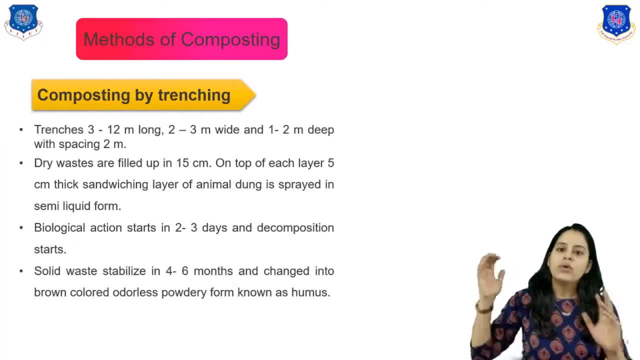 is composting by trenching. So how it is done. So for the that, first of all the trench. the size of the trench, are that right? Then it is 3 to 12 meter long, then 2 to 3 meter wide. 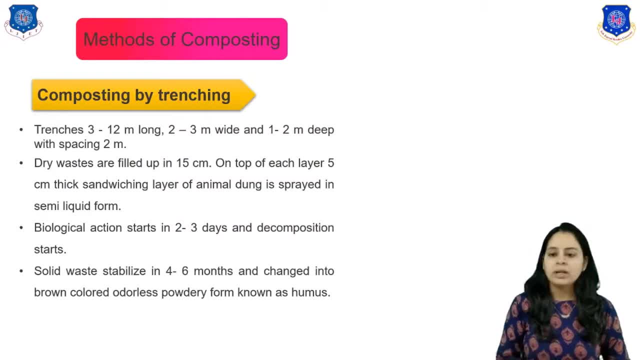 and 1 to 2 meter deep, and the spacing, which is 2 meter right, So the dry waste are filled up into the 15 centimeter. then on top of each layer it is filled up into the 15 centimeter. 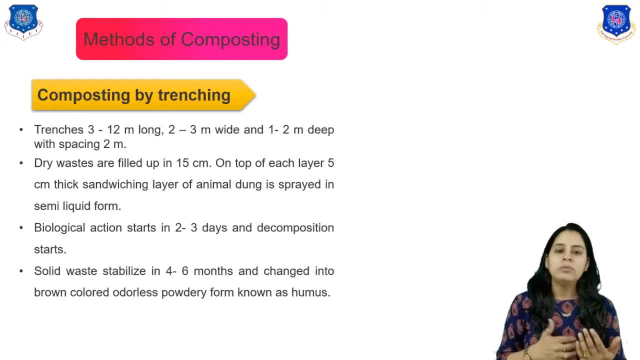 5 centimeter thick sandwiching layer of the animal dung is sprayed on the semi-liquid form, Then biological action start in 2 to 3 days and the composition decomposition will be started. Then solid waste, which is stabilized in 4 to 6 months and change into the brown color. 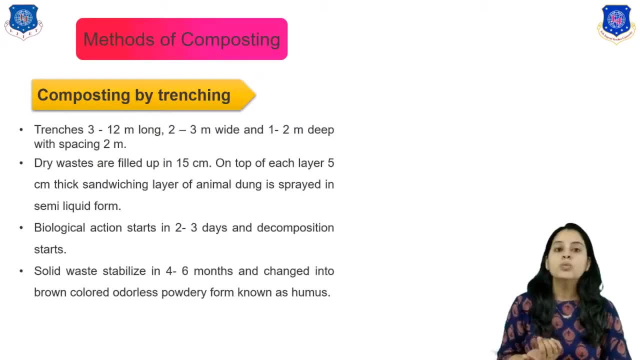 or the less powdery form, it is known as a humus right. So here on screen you can see that, the examples or the figure of the composting. So here on screen you can see that, the examples or the figure of the composting. So here on screen you can see that the examples or the 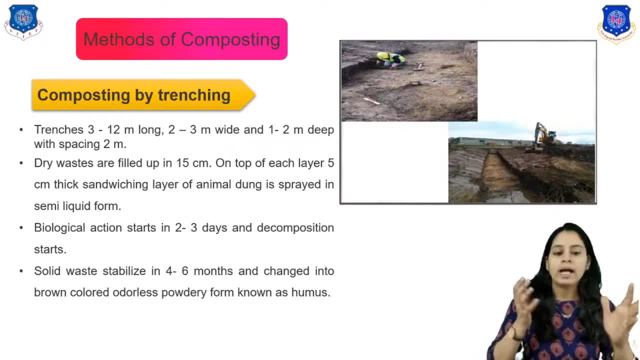 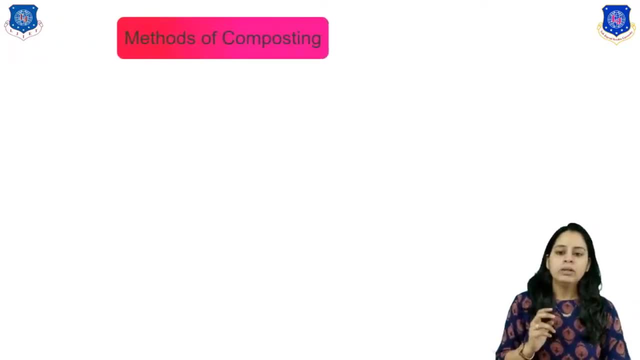 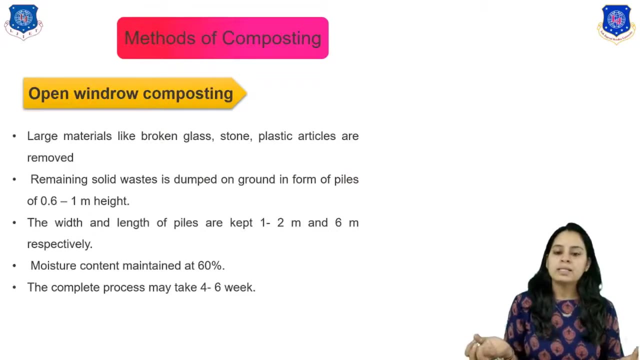 figure of the composting by trenching. are that here? You can see that the trench for the composting method, the trench. are that right Now? the second method, which is open withdraw composting. It means that the large material like broken glasses, stone, plastic, 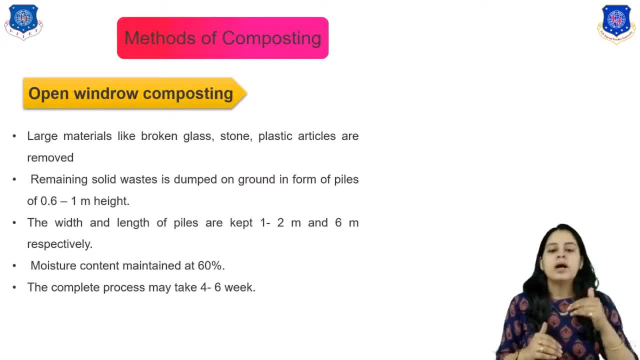 articles are removed and remaining solid waste is dumped on the ground in form of the piles of 0.6 to 1 meter height right. The withdraw composting method is called as open withdraw composting. The withdraw composting method is called as open withdraw composting method. 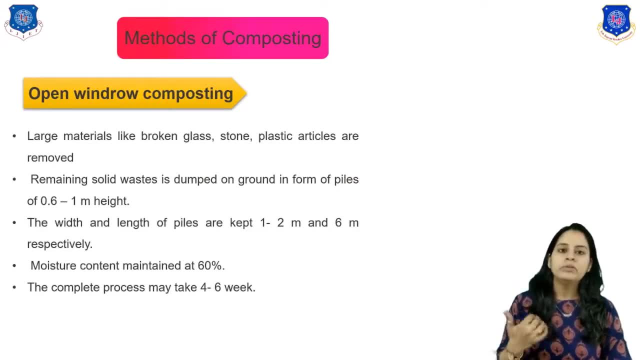 Right. The width and length of the pile are kept, with width 1 to 2 meter and 6 meter respectively. Then the moisture content is maintained at 60% And the complete process we take a 4 to 6 week right. Okay, Here on screen you can see that the open withdraw composting method. 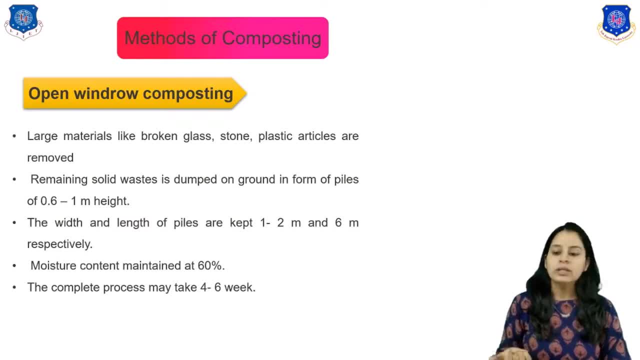 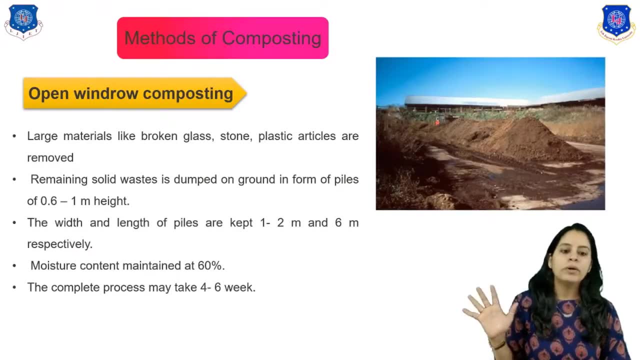 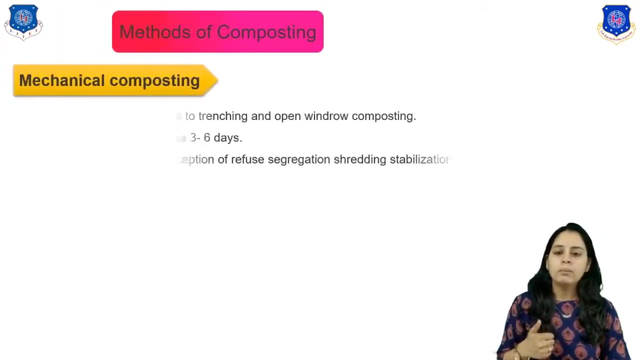 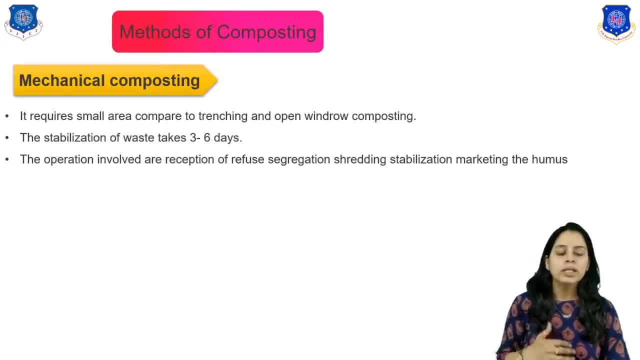 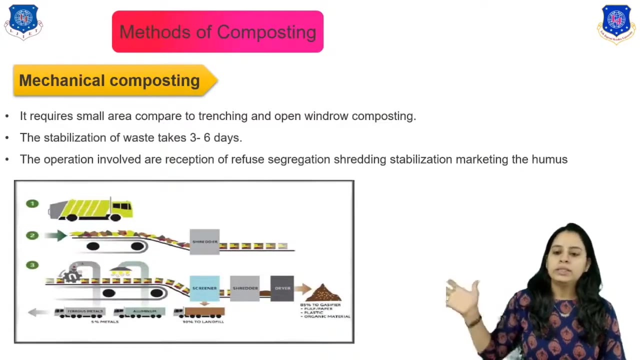 stabilization of waste, which required three to six days and had the operation involved in the reception of the refuse segregations writings, uh, stabilization and the marketing the right. okay, so here on screen you can see that the mechanical composting method are there, uh, for in this mechanical composting, the operation which is this aggregation and 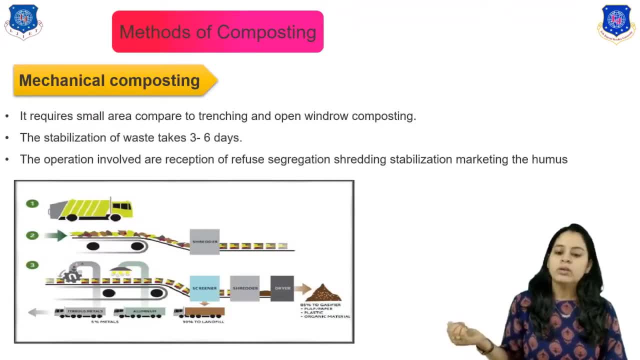 threading. okay, then stabilization. okay. so for this, for the segregation purpose, we are using belt conveyor. okay, for here on screen you can see that the belt conveyor used for the segregation of the waste, right? okay? so this is the first method, which is composting method. right now the second. is also called sanitary landfilling right. so a land filling site is a site for the disposal of waste material by murray and it is the oldest form of the waste treatment right. so the, in this matter, waste is directly dumped into the- uh, my new poets, or the boropets right and the disposable waste. 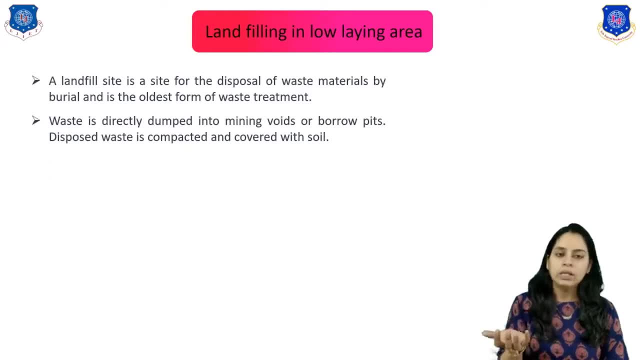 is compacted and converted with the or the cover with the soil, so the gas is degraded by this matter. this waste material are often burned to regenerate power and the landfilling can be done by the three: math or the trench method, area method and the third one, which is gram method. right, okay, here the modern. 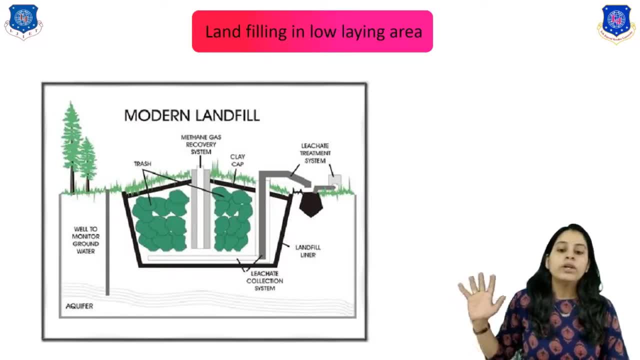 land filling methods are the figure which is given. so here you can see that the clay tap are there, then dresses are there, after that the in land filling method, the leachate which is generated right. so here you can see that the leachate collection system is generated in the leachate collection system. 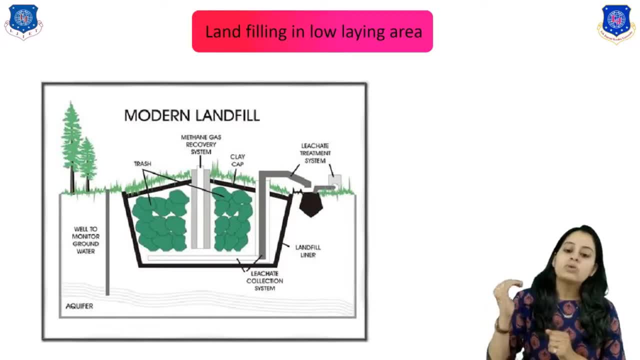 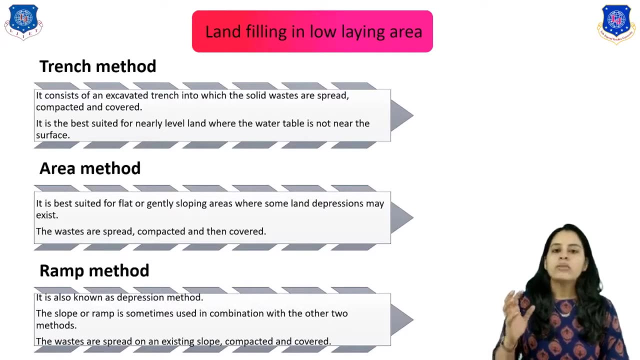 are also given because this leachate which goes to the ground water, they pollute the ground water. so here the leachate collection method. are there right? ok, so the first method, which is trench method. so it consists of an excavated trench into which the solid waste. 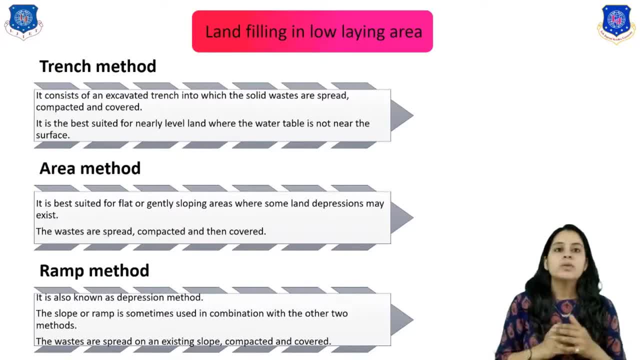 has spread, compacted and the covered. it is the best suited for nearly level land and where the water table is not near the surface. ok, the second method. in this method it is best suitable for the flat or gently slowly ground where some land dispersion may be exist. 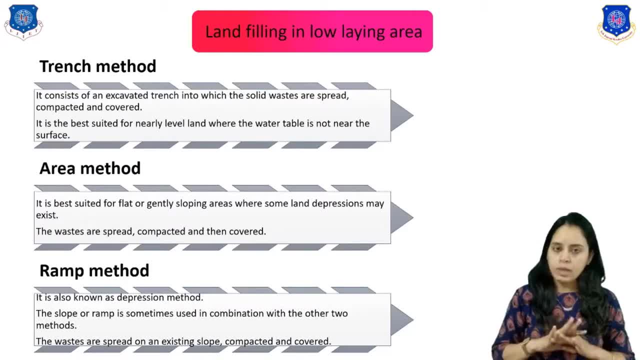 ok, the waste has spread, compacted and the covered right and the ramp method. in this method, it is also known as the depression method- the slope or a ramp is sometimes used in the combination of the surface and the ground. So this is the combination with two method and the waste is again spread. that spread. 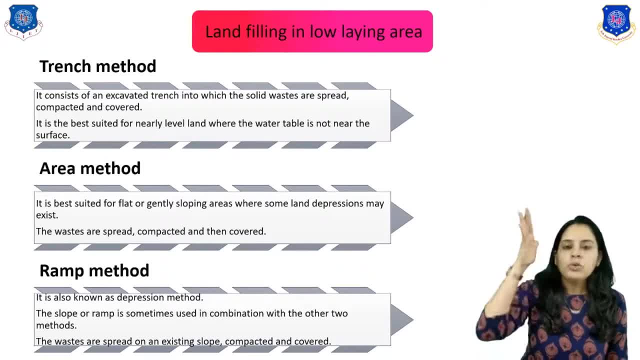 of the existing slope, then compacted and the covered: ok. so major difference between is in three method, which is the place for the trench method, it require trench. then in area method, it is suitable on the flat ground, and the draft method. in this method the slope is required right. so this is the main difference of this three method. ok, advantage of this. 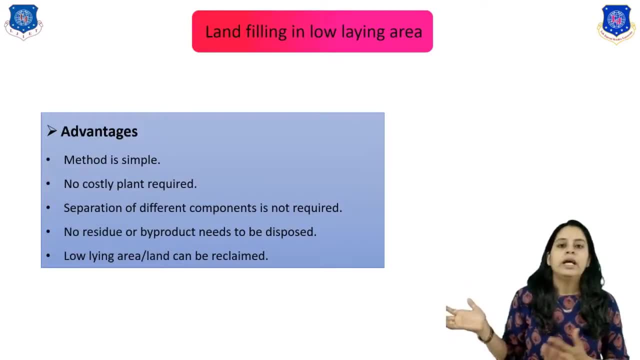 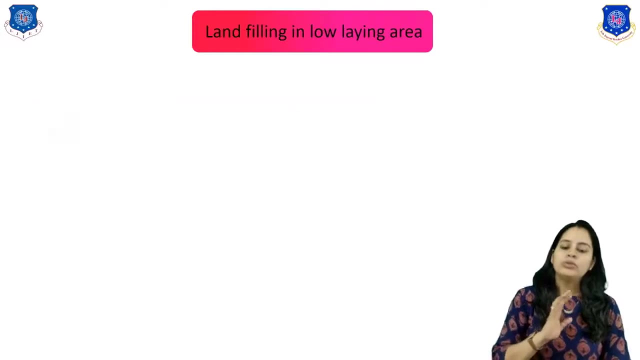 method which is the method is suitable on the flat ground and the draft method in this method is very simple method. then no costly plant which is required, then separation of different component is not required. then no residue or by-product need to be disposed and the low laying area it can be reclaimed right now. so this third disadvantage are also. 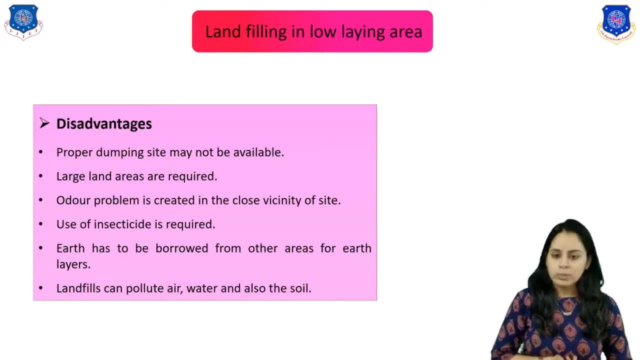 there, ok, so the proper dumping site may not be available, then large length area will be required. then order problem. then use of the insecticides is required. then earth has to be borrow from the other gases for the earth layer and the last, which is land, will it create. 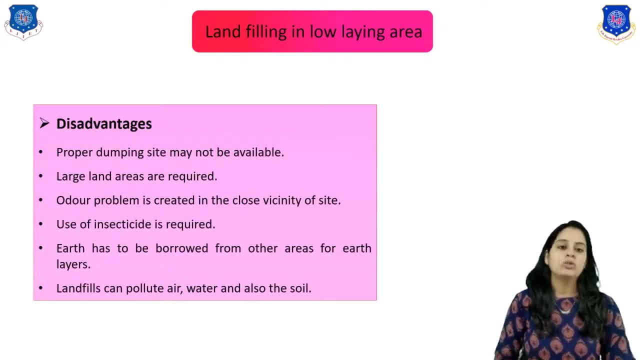 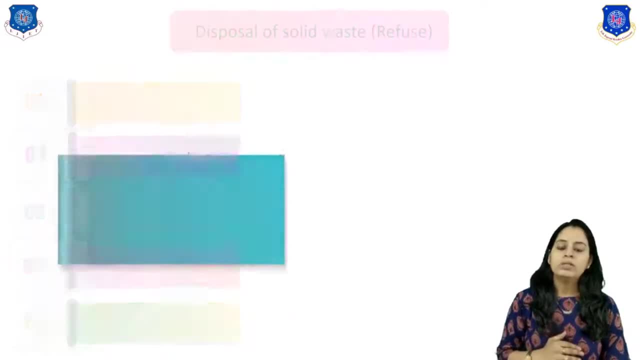 a pollute. it can pollute air, water and also the soil, right? ok, so this is the land relief method. now the third method, which is incineration method. ok, incineration method. it is a waste management technology that involves the combustion of organic waste material. right, it can be. 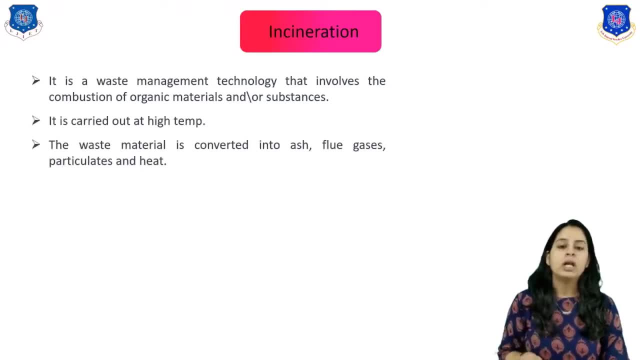 carried out in the high temperature or it required high temperature and the waste material is converted into the airs, then foul gases and the particulates and the heat. ok, the type of incineration, which is a moving grade incineration, then fixed grade incineration, then fludized. 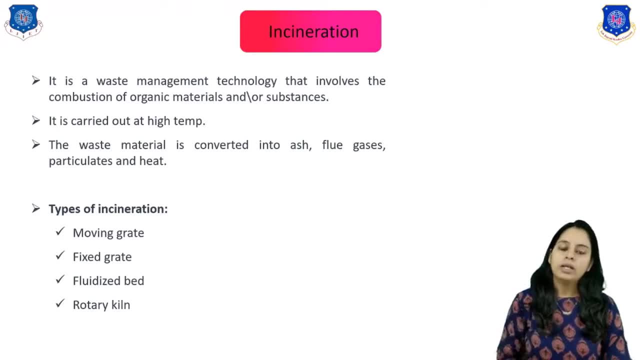 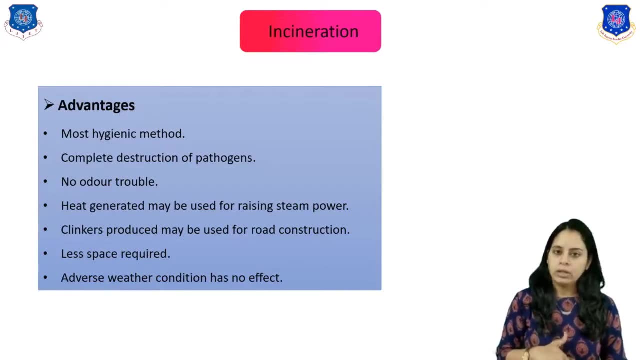 bed incineration and the rust which is in the rotary key right. so the advantage of this method, which is it is a most hygienic method, right. then complete incineration is required. then it can be used for the destruction of the pathway joints, then no order problems. 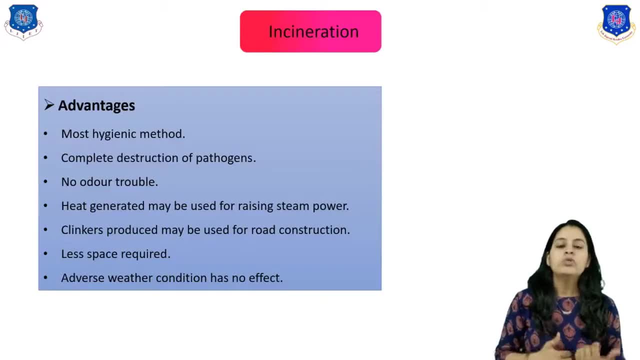 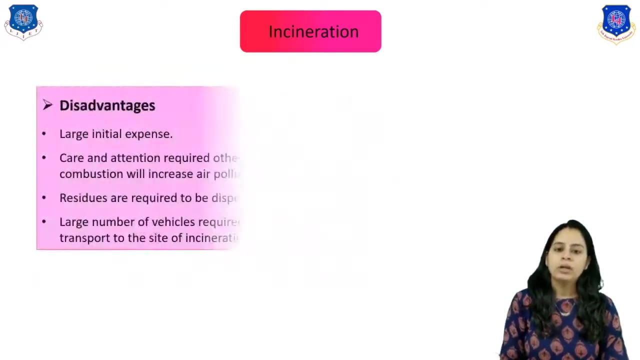 are there. the next is heat generated can be used in for rising the steam power. ok, then linkers produced may be used for the road, road construction also. then less waste is required and the adverse weather condition has a no effect. ok, so there is advantage of this method, which is large initial expense because it required a coxley plant. then can 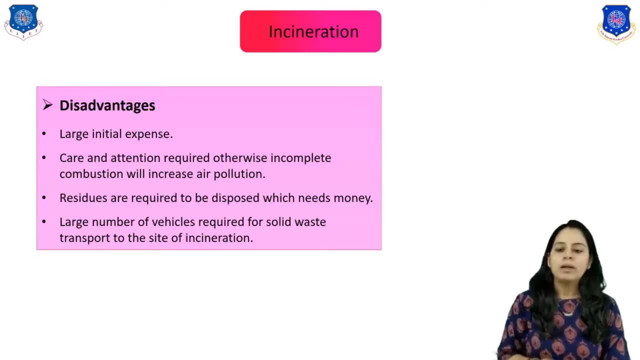 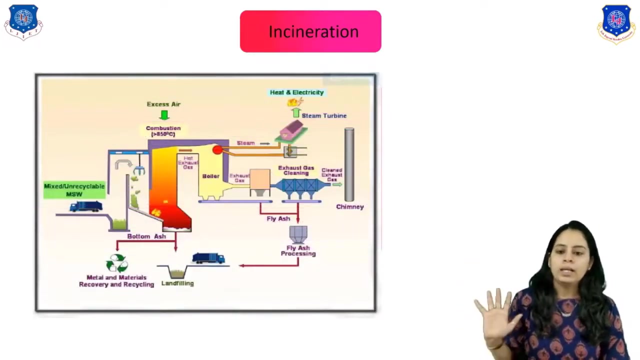 care and attention required, otherwise, in complete conversion will increase the air pollution right. then residue are required to be disposal, which need the money, and the last one, which is large number of vehicle required for solid weight transport to the side of the incineration right. so this is the disadvantage of this process. ok, here the plant are there. basically. 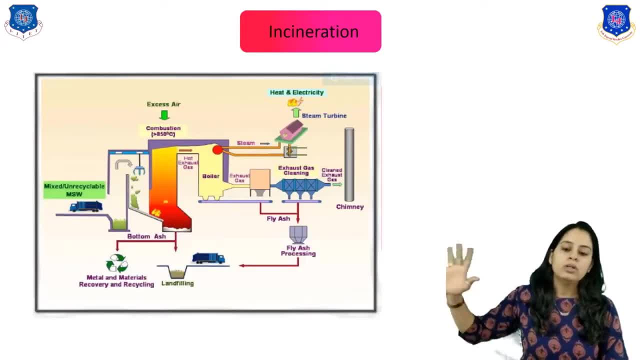 the waste which is goes to the. here on screen you can see that the waste is going to the waste which is transported and the soft waste, whole waste which is storage in the container. after that, some part of the waste which is goes to the combustion process and some part 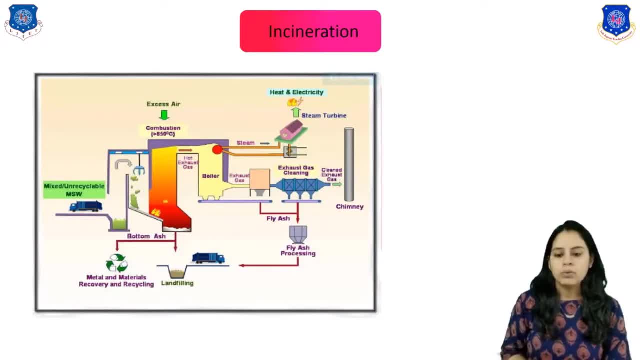 of the waste, which is goes to the recovery and recycling process, right and the combustion process. the waste, which is the combustion, and the air, the excess air, are the heat will be produced and this heat will be used in the boiler to generate the steam. right and the last one and the some bi product residue product are also generated, which is as and 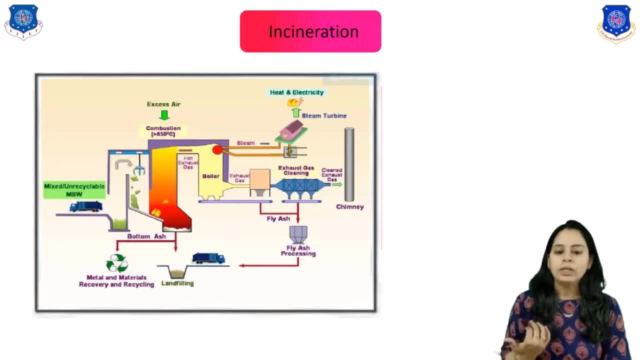 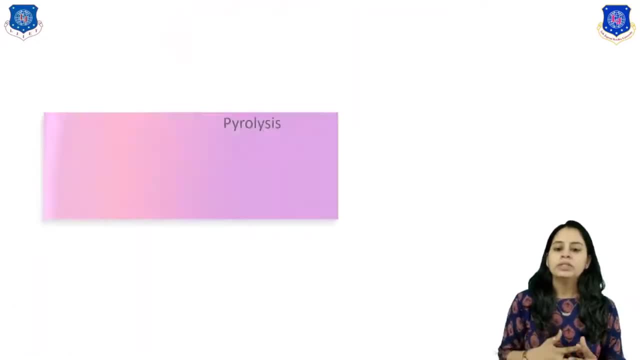 these bi product which goes to the land filling process. right, ok, ok, so this is the all about the incineration process. now the next one, which is the pyrolysis. ok, so what is pyrolysis? it means that it is the same process, same as the incineration process, but it is a thermochemical 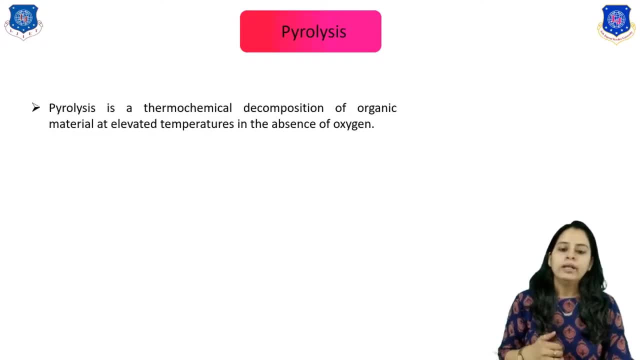 decomposition of our air right. So this is the process of the pyrolysis, which is the process of the pyrolysis of the organic material right in absence of the oxygen, and it required temperature about 1200 degree celsius to 1000 degree celsius. it involves the simultaneous change of the chemical composition. 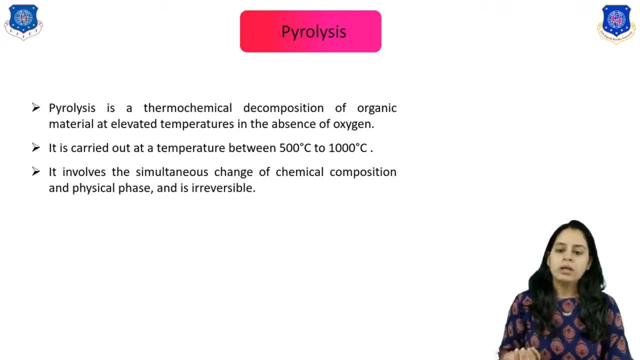 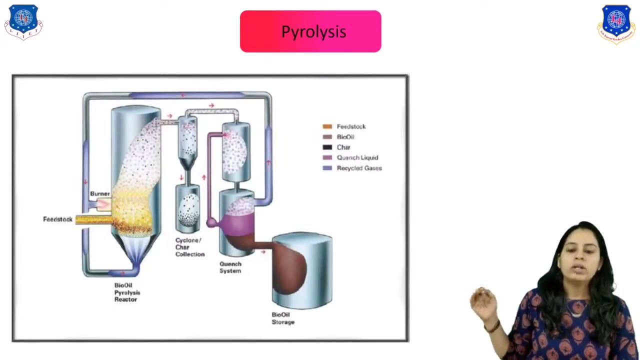 and physical phase and it is irreversible. right and external heat source is employed and it killed gaseous and liquid and solid reactions. ok, so here on screen you can see that the plant of pyrolysis are there. ok, The first of all, the material or solid waste which is inserted or goes to the pyrolysis. 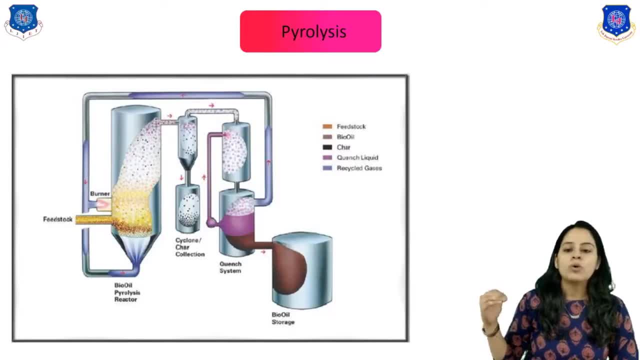 process, pyrolysis process. then external heat is provided and the temperature will be 500 to 1000 degree celsius after that, which is heat is generated and the for cleaning process. here the cyclo separator are used for the cleaning the process right.